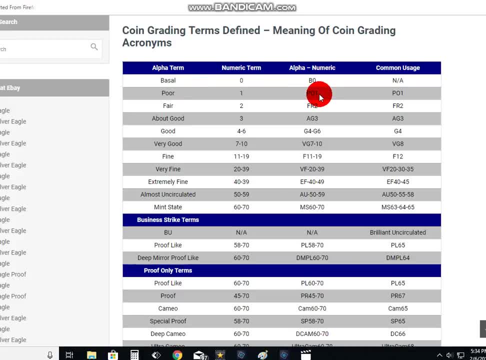 Poor would be the lowest you are going to see on a holder And that's PO1.. When we combine the alpha and the numeric together, it's called alphanumeric And we have fair 2, AG3, G4, G6.. 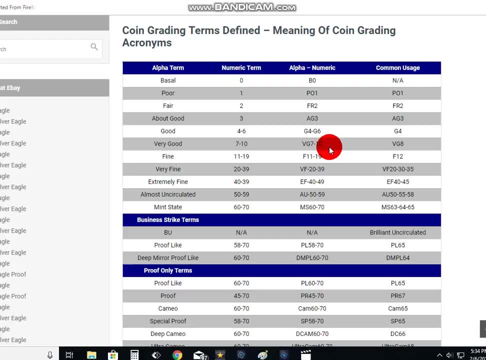 These are grades that you do see. We don't use all the numbers. We don't use VG7, for instance. We use very good 8 and very good 10.. Down, almost uncirculated, you've got anywhere from 50 to 59.. 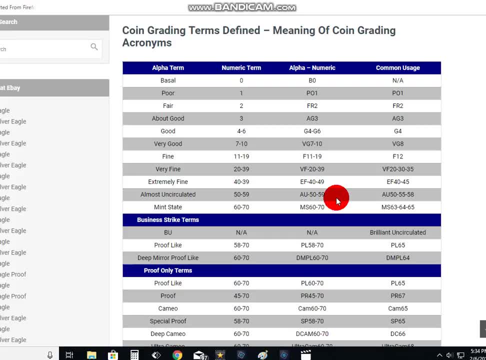 Obviously, we don't use all those grades. We use 50. Sometimes you'll see 53.. You'll see 55. And you'll see 58. You rarely ever see 59. And they call those coins the sliders, because they can go either way. 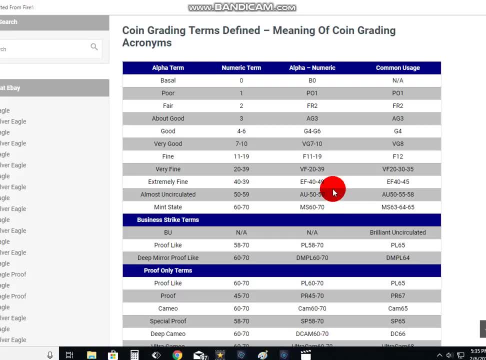 Sometimes the wear is so imperceptible that they kind of err on the side of caution, it seems, And they'll grade them an AU58.. Also, mint state is a coin that's not circulated. It is never circulated. It might have marks all over it. 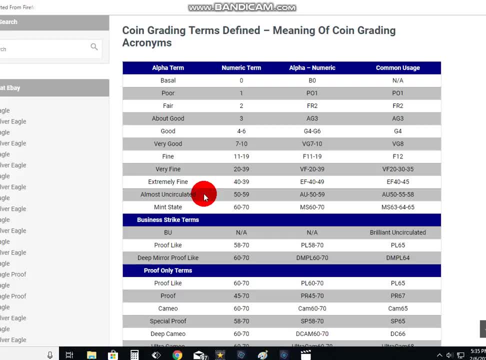 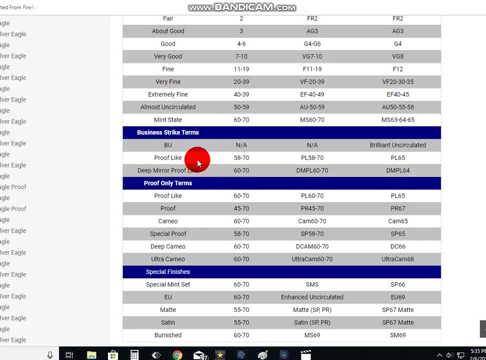 but that will never make it almost uncirculated, Because almost uncirculated is a coin that has a little bit of circulation to it. Here's some business strike terms: Proof-like deep mirror BU BU is another one you'll see on holders. 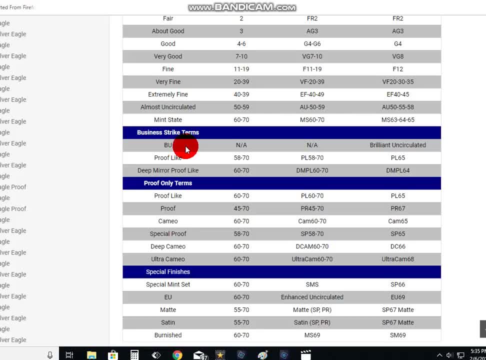 It's not a grade, It's still an alpha term. It's a generic term to describe a coin's condition where it is brilliant but it is uncirculated. Typically that's anywhere from 60 to 70 in the mint state. 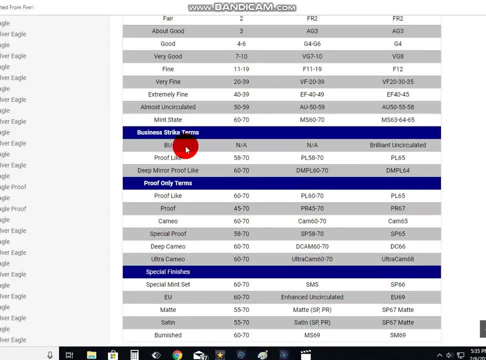 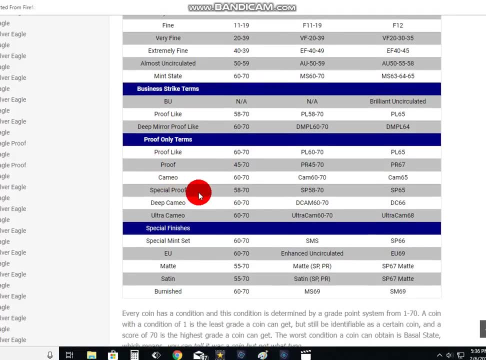 ranges A mint state coin. It is a coin that's at least MS60, and it can go up to MS70.. So that would pretty much be a generic term for that. Also, any of these proof cameo, special proof, deep cameo. 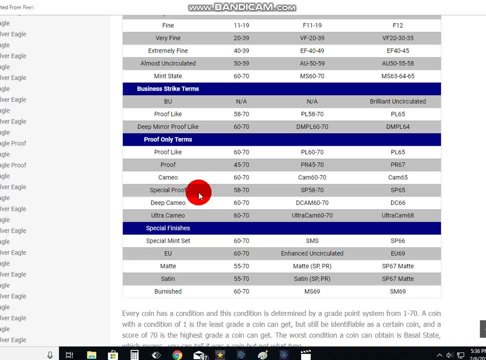 reverse proofs. they're all finishes. The dyes are a special finish, The coins were struck differently, They were struck more than once And also some of the design elements are different, And that's usually apparent Whenever you start examining the proofs. 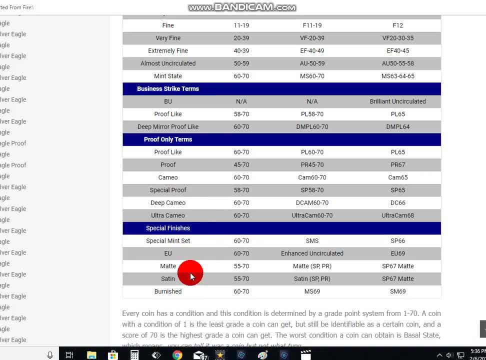 you'll see the differences. Also. you've got some special strikes down here And you have matte finishes, satin finishes, Or you have some special finishes. You have the enhanced, certain circulated in the matte and the satin, And a lot of you have heard of those. 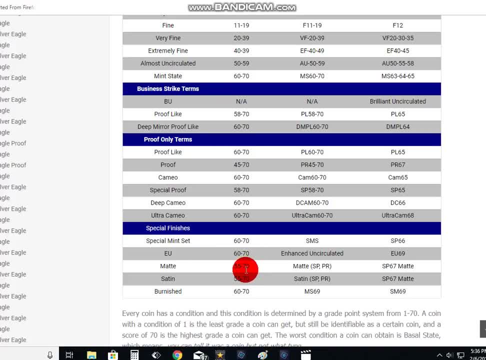 But those are just the alpha terms. So then when you add it to the numeric and you have a coin that is, let's say, SP or SMS55, SP or PR- Sometimes you'll see those kind of terms- interchangeable- EU69 for an enhanced uncirculated. 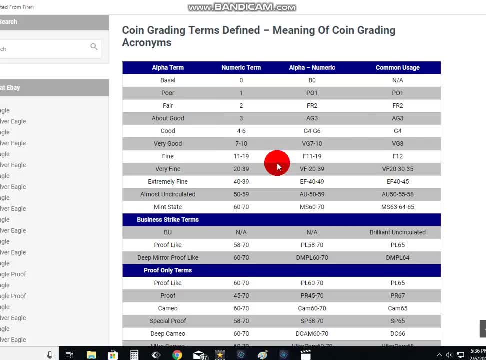 And those are just some examples So you can look at this chart, You can come back to it for reference at all times, You can write it down, print it off. So let's take a look at a few of these and what they actually look like. 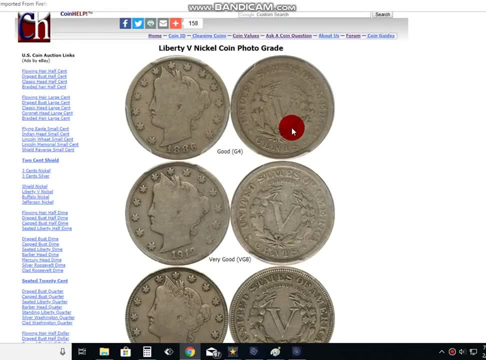 Now also, when you look at this chart and you see, let's say G4. And you know that's good, Basically good condition And it's on four on the Merit chart. So here's Liberty-Nichols. 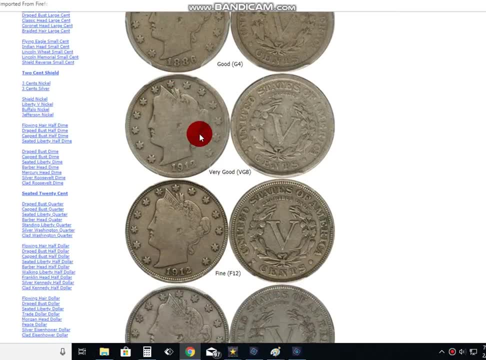 You go down through here and you can see all the terms and what they look like. So at this point you can associate these grades with a picture Of what the coin should look like, And to me that's one of the best ways of grading. 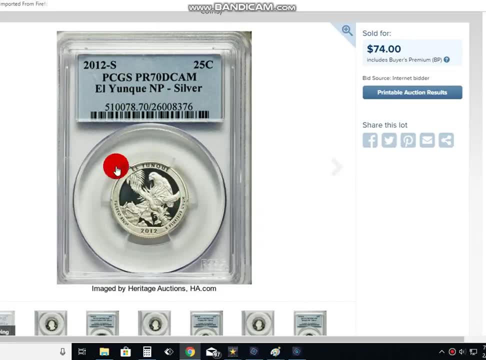 Also, we can see some examples of deep cameo coins. This is a PR decam. As you can see, the fields are mirror-like. The rest of the coin is frosty. It's etched. The die is etched so that it imparts. 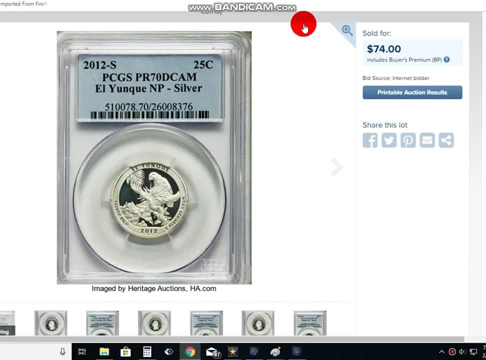 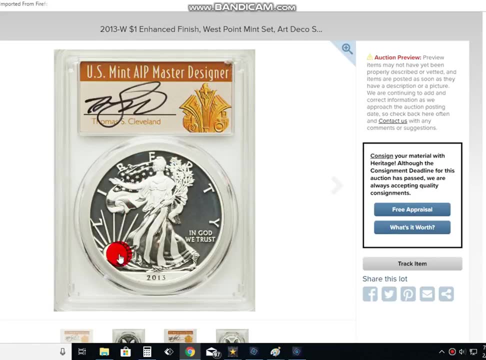 kind of a graininess to it, Brings out some luster and a lot of reflection. Over here you have the enhanced finish And this one is what they. It's a silver eagle. It's a really nice coin on that. 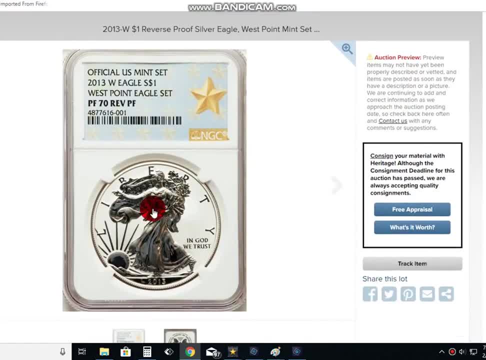 And then you have what they call the reverse proof, Which usually you have the frostiness here, But now you have it in the fields, And then you have the mirror finish on the actual design elements. So I hope this helps you And the best thing to do instead of going through all. 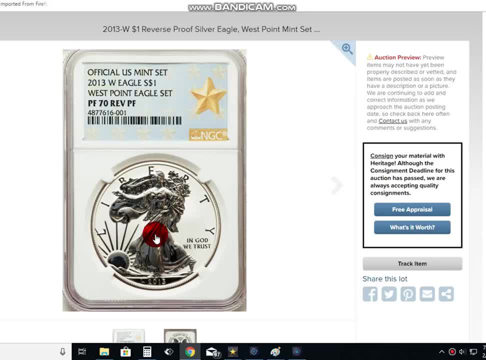 these terms and defining all of them is to go to my website, coinoxioushelpcom, and look up the chart. The next thing that I'm going to do this is going to be a two-part video. I'm going to do the variety and error terms that we use.